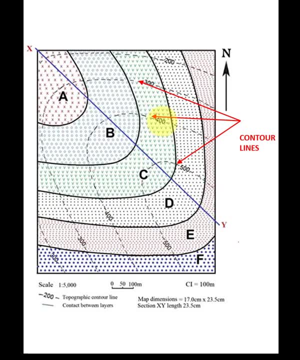 certain terminologies here. So these dotted lines that you're seeing, with the represented, with the numbers, these are your contour lines. and what are contour lines? Contour lines are those lines which join equal elevation. So all the points on this contour line, let us say of this 300. 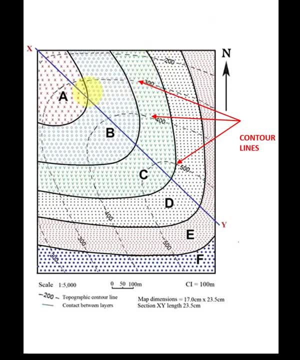 all the points on that contour line will have same elevation of 300 from a particular base base. okay, like we can consider one, maybe sea level we can consider as a particular base, from that we consider heights or any other reference point. Second, after contour lines we have these bedding planes. So in earth science, 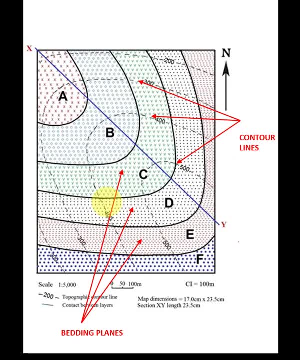 you all had studied sedimentary rocks. so you have. you have also studied that majority of the earth is composed of sedimentary. So here we do have the bedding planes and you know how the sedimentary are made up of different layers. so we have this ABC, and D, E and F. we have 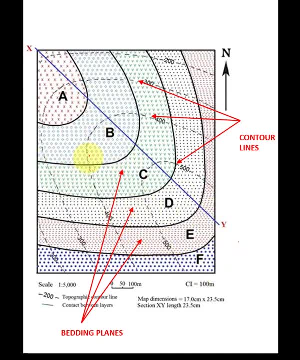 named those layers and on these are your bedding planes. bedding junctions are nothing but the junction between two bedding planes. okay, so these are the three important terms that we need to understand before solving it, and also, what you need to see here is the scale of the map. so this thing you need to. 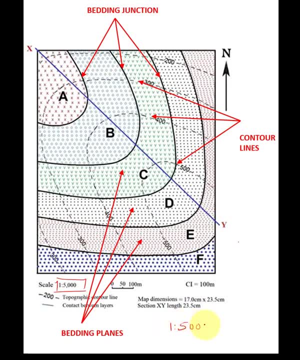 remember, the scale is given as 1 is to 5000. we'll be doing certain calculations, so for that we need the scale and also the contour interval, which is 100 meters. so contour interval is nothing, but the interval between every contour is like you can see, it is 200, then after the 300 we have drawn, then 400 is there and then 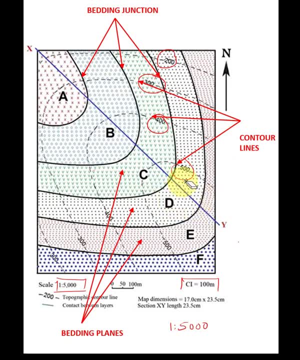 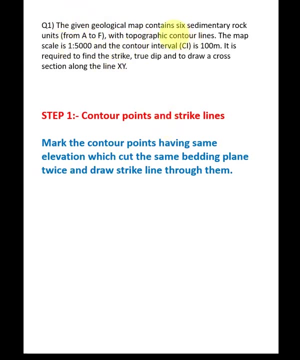 500 is there. so only for these particular contour heights the contour levels are shown, shown in this map. this is what it means: contour interval. so let us see the first step of it. the question is that the given geological map contains six sedimentary rock units, from A to F, with topographic contour lines, the map scale. 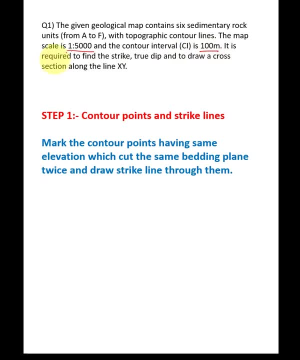 is 1 is to 5000 and the contour interval is 100 meters, it is required to find the strike true dip and to draw a cross section along the line XY. and before going into the calculations, I'll tell you that there are four maps that we'll be solving. the PDF of those four maps I'll be giving in the 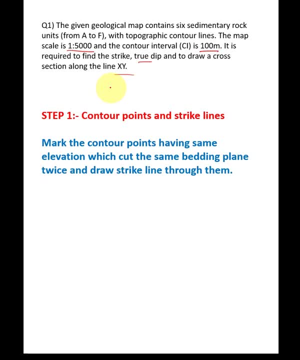 description of this video. you have to download those maps, you have to take a printout, you will have to do what we are doing in this video tutorial. we'll have to do it by yourself and then you have to submit that. okay, fine, so step one is to draw this 2-way contour without drawing the flat geek. 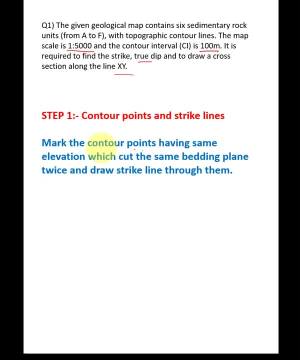 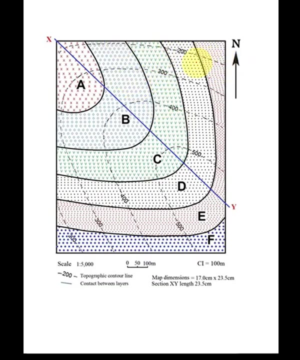 this says is contour points and strike lines. we need to mark the contour points having same elevation, which cut same bedding plane twice, and draw strike line through them. so now, what we essentially need to do here is that we need to consider one strike, one contour line first, and 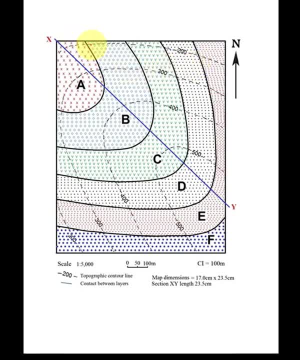 we need to see that where that contour line cuts two bedding junction means cut cuts a bedding junction at two places. okay, for example, this 300 contour line which you can see, it is cutting the bedding junction bit between the bedding plane a and b. so i'll call this bedding junction as a- b. 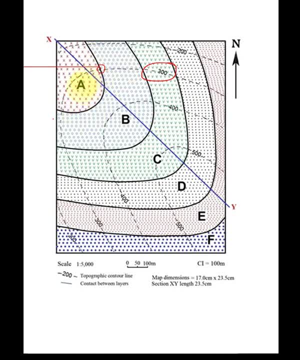 okay, so it is cutting the bedding junction a- b, first at this point, second at this point. right, so we need to mark such points. okay, so these are the two points where this 300 uh contour line is cutting the bedding junction a- b. when we join these two points, we get a strike line and we will name that strike line immediately. 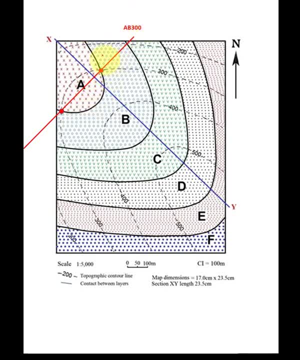 so what we'll say is that we will write the name as a, b, 300. it means that it is cutting the bedding junction a, b and which contour is cutting- 300 contour is cutting okay. so this is the idea that we are going to proceed with. similarly, let us see that. uh, what? which other points are there? so you? 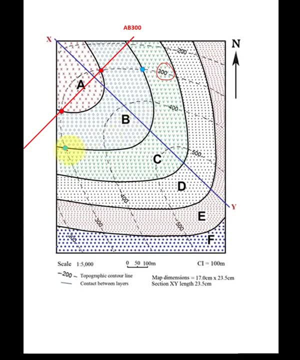 can see that this 300 mm contour is cutting this bedding junction bc at this point and this point. so we'll pass a strike line, i mean, we'll connect them and we'll get one more strike line, right. so this strike line, we'll name it as bc 300 because it is cutting the bedding junction bc. 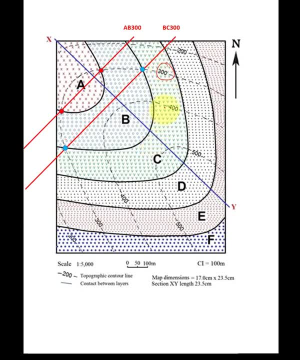 and 300 is the one which is cutting it. next we have this 400 contour which is also cutting your contact point. so again, a strike line needs to be passed through it and that we will name it as bc 400, because it is cutting the bedding junction bc also. this can also be named as cd 300. 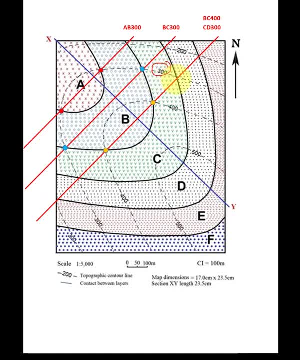 because this same strike line, you see, this 300 mm contour, is cutting at the same two points through which this strike line is passing right. which bedding junction it is cutting. It is cutting CD junction right. So this same strike line can be named as CD 300 also and BC 400 also, and you have to name one strike. 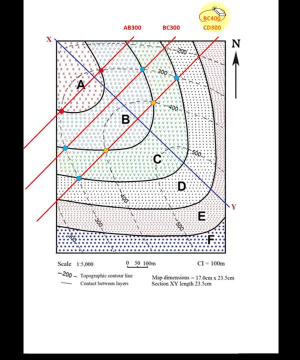 line with as many names as possible, right? So, for example, here I have only named it as AB 300 or here only BC 300, but we can see that it is not only BC 300, but this 200 contour is also cutting this junction. Sorry, this 200 contour line is also having a point on. 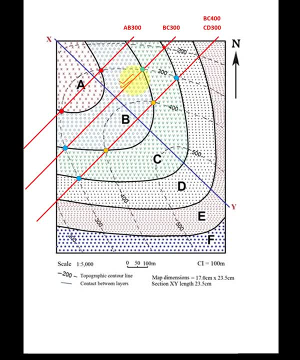 this junction CD which is lying on this strike line right. So we will see that later on how to find the missing strike lines, But first just understand what is the concept that we are following here. After 400, we will see which other points. 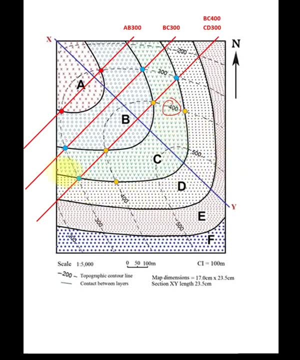 we get. So this 400 contour is cutting your CD junction at these two points, right. So we will draw a strike line through that and this strike line is named as CD 400 and DE 300 will come on that. So DE 300 because on the same strike line. you can see that here there is one point. 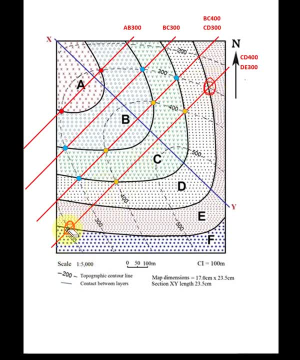 and here there is one point which is being cut by, sorry, not this point. Yeah, yeah, this point. and this point which is being cut by 300 mm contour, Not mm 300 contour line, right, So? and this 500 contour line, here it is cutting your CD junction. 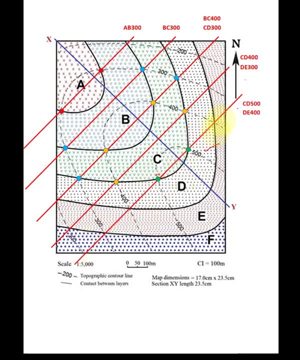 at these two points. So we will pass this strike line through them also and this strike line will be name as CD 500 and DE 300.. de 400 de 400 because this 400 mm contour line is cutting this de junction at this point. 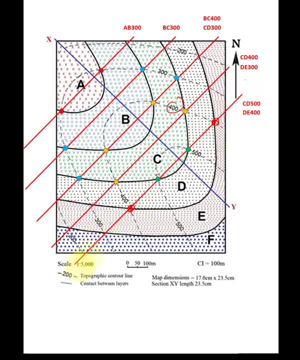 and this point and these two points are also lying on that strike line itself. yes, so these are the names that are given. further, this 500 contour is also cutting this de junction at these two points. so again, we'll pass the strike line through them and it. 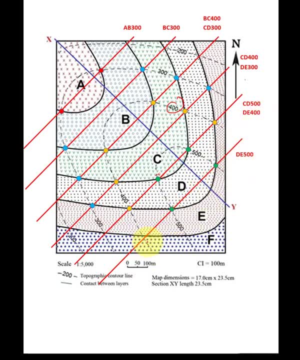 will be named as de 500. now, after we have named these strike lines and drawn the strike lines, what we can see is that the nature of the strike lines are parallel to each other. all the strike lines are parallel to each other and when you draw it on your map, you will also see that all strike 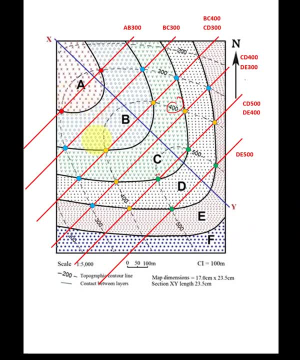 lines are placed at equidistant, so you can see that all the lines are placed at equidistant, so they are equidistant from each other. this is the nature of the strike lines that you have to remember. okay, from this nature we can get some more strike lines. 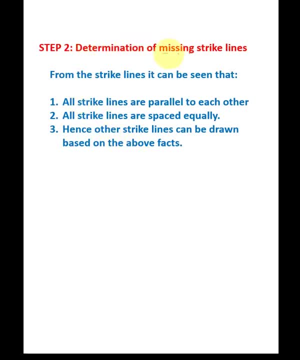 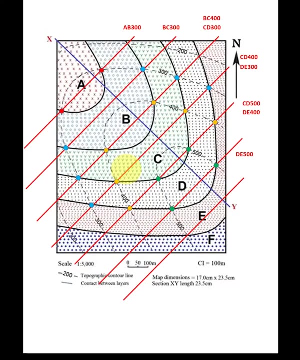 so we will find that. so the next step is determination of missing strike lines. and from the striking it can be seen that all strike lengths are parallel to each other. all strike lengths are spaced equally, hence other strike lengths can be drawn based on the above facts. so how we'll draw this? 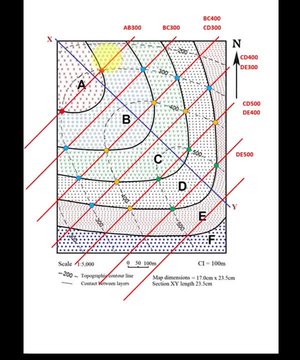 at first. see, you can see this 200 mm contour- sorry, 200 contour- which is there. it is cutting your a- b junction at this point, right, but the other side of the contour is not shown in this map. but we can safely assume that this contour will go something like this this: 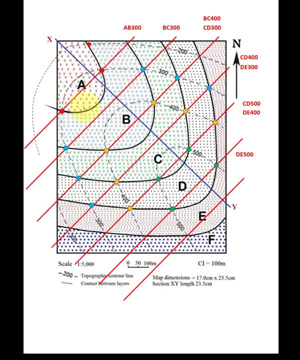 way, how it is shown here, and that missing strike line would be like, if I just extend this a, b junction ahead, I'll get my missing strike line, which would be parallel to your other strike lines, also equidistant from them, right? so one important tool that you require. 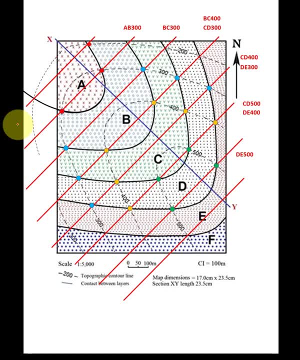 while drawing these maps is your roller scale, because by roller scale you can easily draw parallel lines. obviously, drafter, you won't be means for such small thing, you don't need a drafter, but with the roller scale we can definitely draw parallel lines. so this is one of the missing strike line and what it would be. 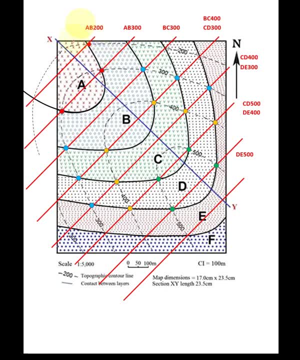 named as a b 200 because it is cutting a b junction and it is being cut by 200 contour. next, if I extend this b c junction like this, okay, then what I'll get is again you see that this 200 contour line is cutting strike line here once. 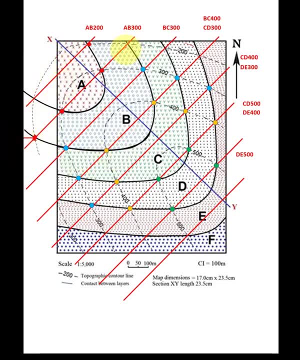 and the same b c junction. it is cutting here as well, so this a b 300 can also be miss this strike line, which was named as a b 300. one more name would be added there, which is b c 200. right, we need all the different types of names possible for a particular strike. 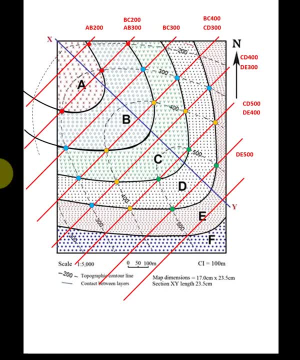 line, because that is important in drawing the map. the next, which are the strike line we can draw. so you can see that here in this strike line it is having a point which is being cut by 200 contour, but on the other side we do not have the 200 contour meeting. so you can see that this contour line will go like: 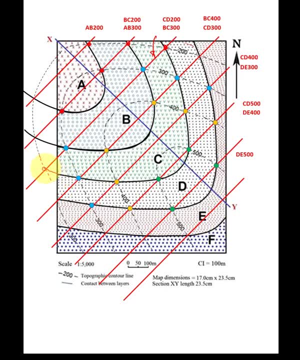 this and this C, D junction will come up like this: so this is the other contour point where it is meeting that junction CD, right? so here, once it is cutting the junction CD, and here, once it is cutting, therefore, this strike line will also be named as CD 200. okay, then we. 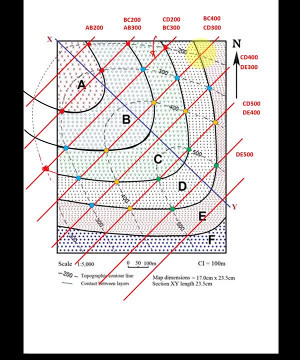 have this here: this junction DE is being cut by 200 contour and on the other side you can see that this is a 200 contour which this contour line would have extended this way, like this, that contour has to come throughout, okay, it has to come all the way this way, and 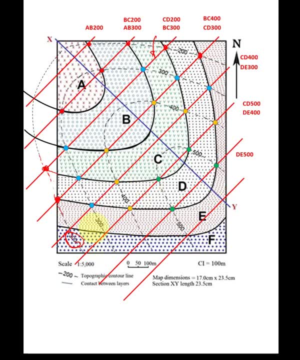 then it would cut your junction DE at this point somewhere, right, roughly at that point. so again, this strike line would be named as DE 200. also, right, DE 200.. Okay Then which other strike line is there? So your this 200 contour is cutting this strike line, cutting the EF. this 200 contour is cutting. 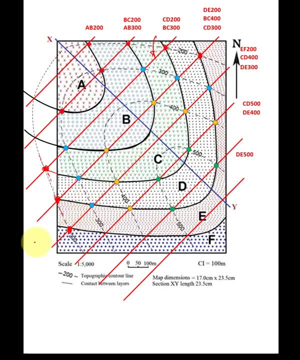 the EF here at this point for this, for this strike line, okay. on the other side, If this EF was extended somewhere like this, it would have meet the 200 contour on the on that same strike line. so probably you are getting what what we are doing, exactly right. 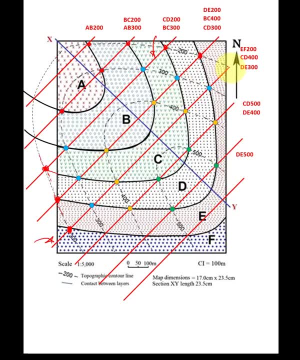 the strike lines would be parallel, they would be equidistant as well as this contour. if it is cutting on one side- definitely if it is not shown in the map- it will cut it on the other side as well. So we can assume this and we can say that this strike line 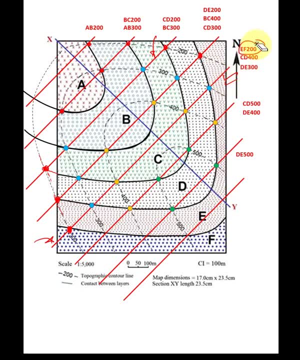 Is being is can also be named as EF 200. further, this 300 contour is cutting your EF at this point, right. similarly, if EF was extended this way, let me just use some other color. so this: if this EF, Okay, Okay, Okay. So if we are extending it, 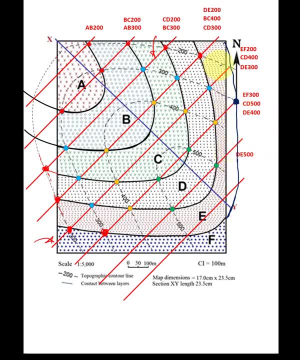 Like this. then you can see that this 300 is being cut here on the same strike line and hence that this strike line can also be named as EF 300. then ahead, what we have is this 400. you can see it is cutting it here at this point. 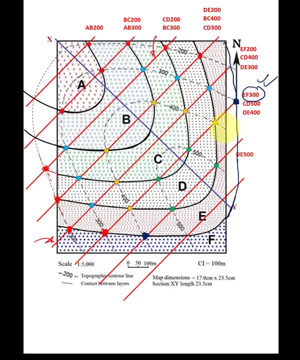 On the other side where it will cut. On the other side you can see that this 400, if I extend it, is cutting on the same strike line and hence this can also be named as EF 400, because it is cutting the junction EF and 400 is the one just cutting it right. and this 500 is also cutting your EF here. and 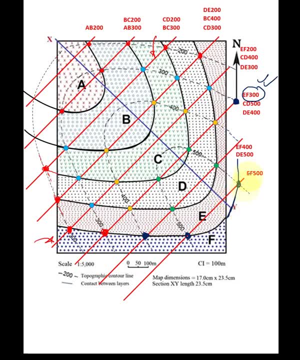 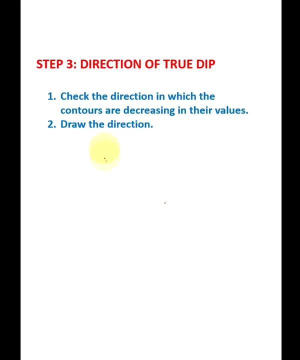 if I extend this 500. It will cut. It will cut this strike line so it can be named as EF 500.. So next step is we need to determine the direction of true dip. so in this we need to check the direction in which the contours are decreasing in their value and we need to draw that direction. 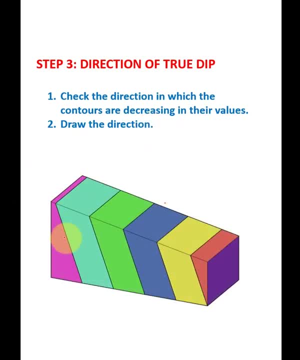 So, as you can see here in this example, I have shown a typical sedimentary rock, and let us say that for every of these planes I Have a certain contour value, for example 500, then 400, 300, 200, that way, okay with a. 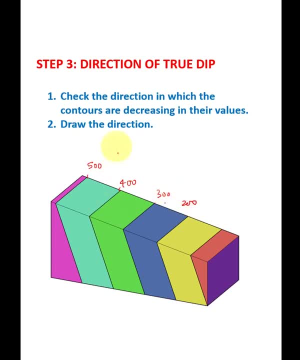 contour interval of 100 meters, you can see that the contour intervals are decreasing in this direction. what this means is that your slope is in this direction, right? so basically, this entire structure is dipping in this direction, that is. that is the only thing that we need to understand. and there is also this word, which is true, so true: dip. if you recollect your 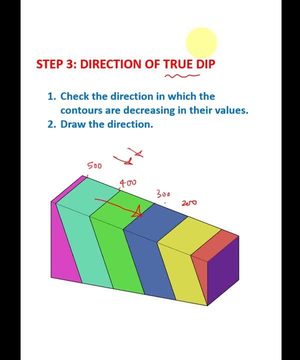 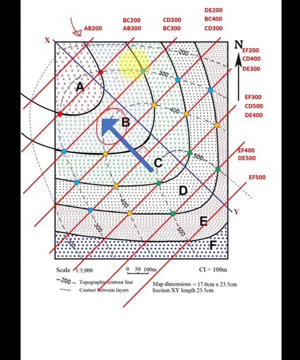 earth science lectures. true dip is the one which is perpendicular to your strike lines. so this direction, what we are going to show, if it has to be a true dip, then it has to be perpendicular to the strike lines. So, in this case, these are your strike lines here and this is the direction of the dip. 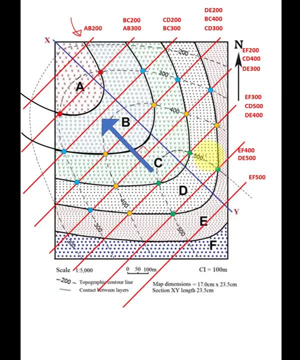 because you see that the contour lines Are: This is 500, this is 400, 300, so the contours are decreasing in this direction. okay, so we understand that the dip direction is that way and we have to also draw it perpendicular to the strike lines. that would mean it is a true dip, okay. 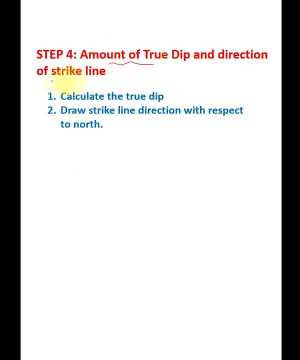 Next is to find the amount of true dip and direction of the strike line. So in this step, what we will do is we will calculate the true dip and we will draw the strike line direction with respect to north. So, first of all, we will draw the strike line direction with respect to north. what this? 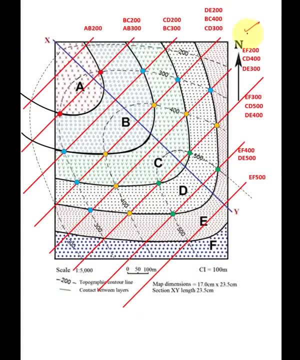 means is that you can see that in this entire map there is also this north, which is shown right. Simply, what we have to do here is which, whatever strike lines we have got in, whatever angle we have to take those, take the angles of the strike lines with respect to this north. okay, 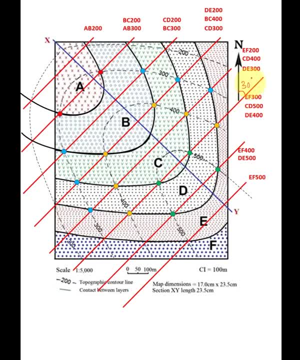 So, for example, this strike line, you get it as 30 degrees. I mean the angle you get with respect to north is 30 degrees. The strike line has to be written as means. the angle of the strike line has to be written as north: 30 east. you might have learned this in serving. or if you want to write it in whole, 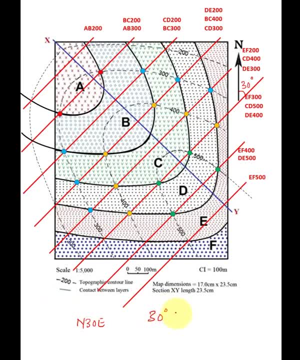 circle bearing. you can also write it as just 30 degrees, that's it okay. Now, this 30, I am just, you know, assuming it. but when you draw it yourself, you will have to take a protractor and you will have to measure that angle. so that would. 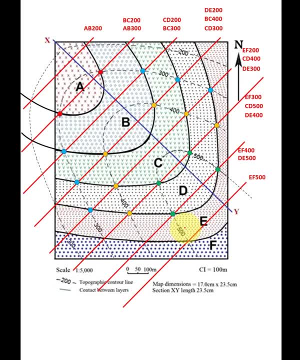 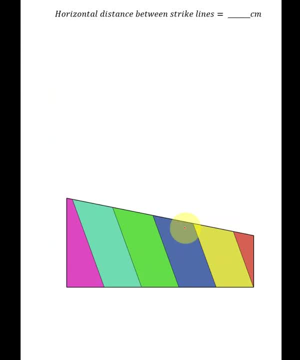 be the angle of your strike lines with respect to the north. next, how to determine the true dip angle. so, as you understand that dip angle, is this one theta? okay, so the way how we will find theta is, let us say that this contour point is 400, this is 300. okay, simply, we'll use tan theta. okay, so tan. 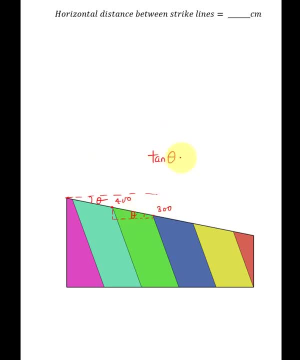 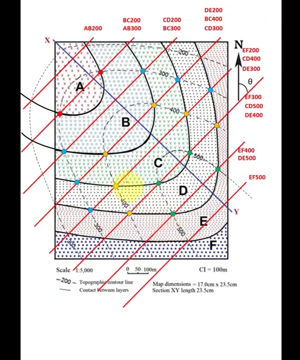 theta is equal to 400 minus 300 upon the horizontal distance between them, horizontal distance right. so how to get this horizontal distance, horizontal distance between strike lines? you will have to measure it on the map itself. so here you will have to take a scale and you had drawn the true dip. 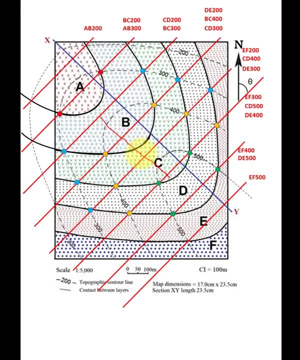 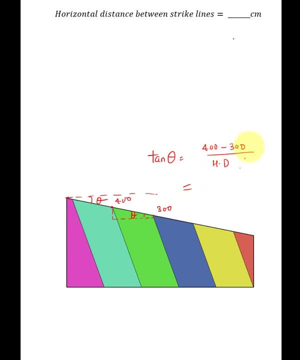 direction. previously it was perpendicular, right, let's say this: is that true dip direction. along this true dip direction only, you will have to measure how much is this distance and that distance you will get in centimeters, correct. so this can be written as this: 400 minus 300. you see, it is your contour interval. yes, your contour interval is set at 100 meters. so 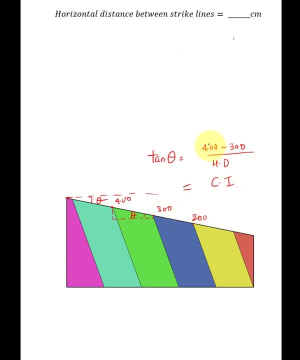 every contour will be like 100 meters apart. so this 400 minus 300 is nothing but contour interval. divided by your horizontal distance, that is equal to your tan theta. fine, this much is clear. now, this contour interval, if you see this, is in meters, but the horizontal distance that you are going to find 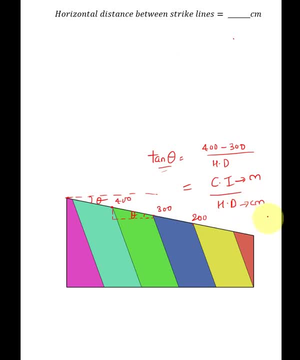 is actually in centimeters. yes, so we cannot obviously use this formula with numerator being in meter and denominator being in centimeter. definitely we cannot use that. so what we'll have to do is that we'll either have to convert the numerator, also in centimeters, or we'll have to convert the 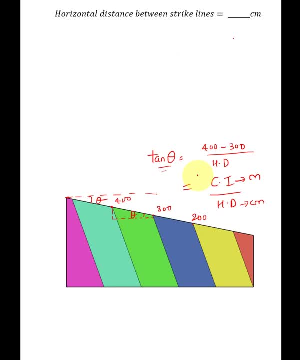 denominator into meters. okay, now one more problem. is there that this numerator is actually the one which is there on the ground, or the denominator is there on the ground, so we'll have to convert the numerator into centimeters. okay, so the denominator is the one which is there on the side, actually, 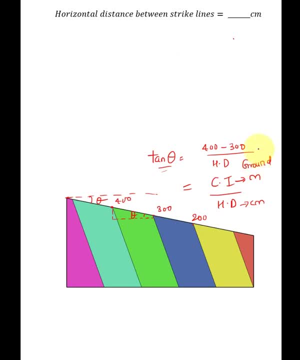 actually on the map. so the numerator is the actual distance on the ground, but the denominator is the distance on the map. so again here there is a difference, right? so what you can do is that let us say that now i am converting the numerator into centimeters. okay, i am keeping both my 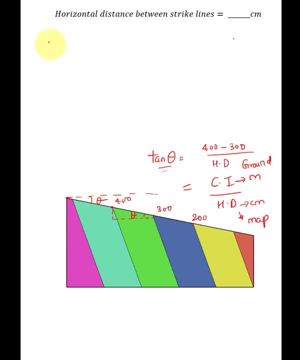 numerator and denominator into centimeters. so now what i'll get is tan. theta is equal to contour interval upon horizontal distance. this was in meters, so if i want to convert it into centimeter i'll have to multiply by 100. right, this got converted into centimeter, but still this. 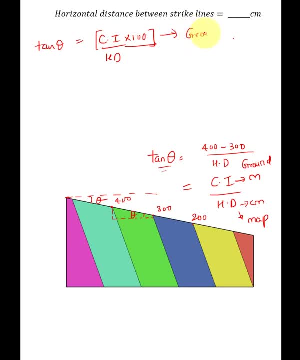 measurement of contour interval is actually the measurement on ground. your horizontal distance is in centimeter, but this is the measurement on the map. if you remember, in the map we had something called a scale. the scale was one is to five thousand. correct what the scale means is. we can also write it as one by. 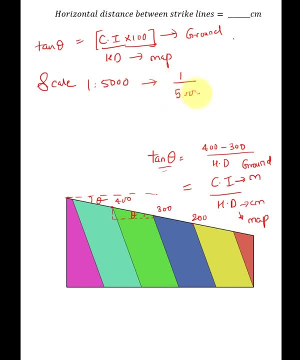 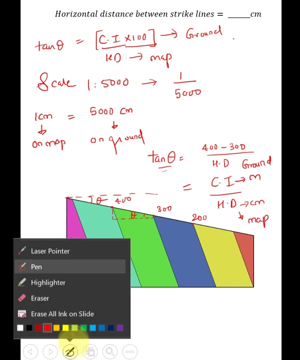 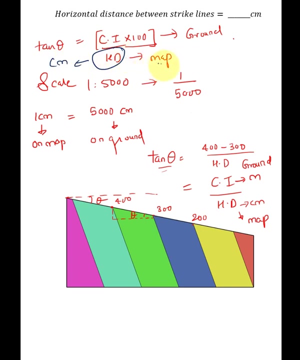 five thousand like this. what the scale means is that one centimeter on map is equal to five thousand centimeters on ground. right hd, okay, horizontal distance. so horizontal distance and multiplied by horizontal distance: okay, so this horizontal distance in centimeters on map is equal to 5000 into horizontal distance on ground. so if i 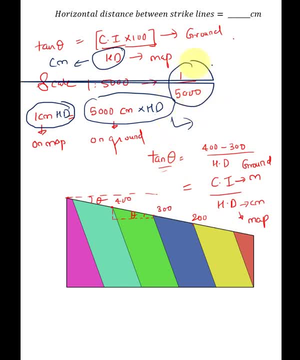 have to generalize this. let us say now see, this is your scale, this is the scale of the map, correct? if i want to generalize everything that i have done here. and ketone tether, tan theta is equal to contour interval into 11. unsettled. its makes this contour interval as centimeter. 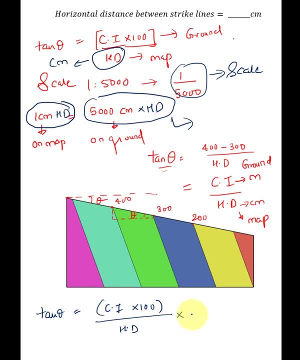 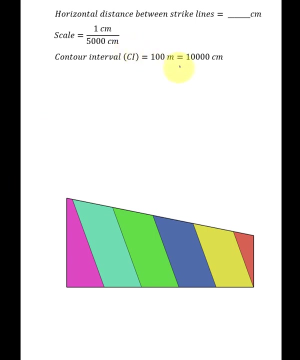 divided by horizontal distance, into scale of the map. what is key? scale of the map is 1 by 5000, so automatically this rituals abundance. get my deeply. 5000. so now everything is fine, will be used in this formula, correct. so this is how Now we will be finding the true dip angle. contour interval is 100m which, if I convert, 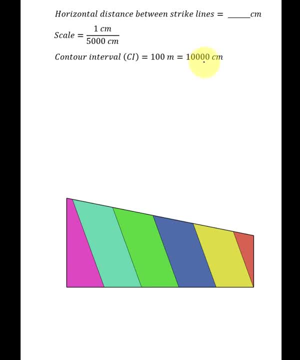 it into cm, it will become 100x100, which is 10. raise to 4 cm. This is on ground. Horizontal distance between strike lines is whatever it is that is on map. To convert from on map to on ground, I multiply by scale. 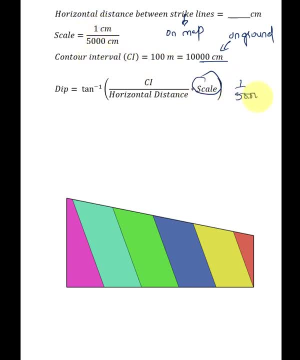 Scale is nothing but 1 by 5000.. So this also, you have to do the calculation, You have to find how much, what is the distance between strike lines on the map, and you have to put it in this formula so that you will get dip theta as tan inverse of contour interval. 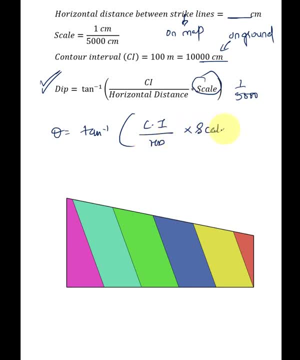 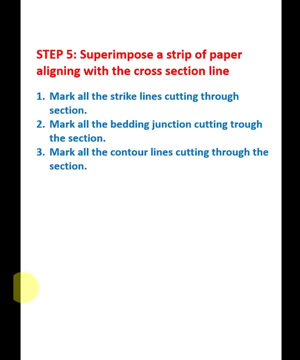 upon horizontal distance into scale. Next step 5 is superimpose a strip of paper Aligning with the circle. Mark all the strike lines cutting through section. Mark all the bedding junctions cutting through the section. Mark all the contour lines cutting through the section. 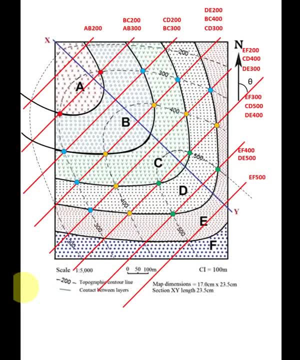 So what you have to do in this case is you will have to take a strip of a paper. You have to tear a small strip of a paper. Let's say: this is that strip you can see here. You have to align this strip along your xy. 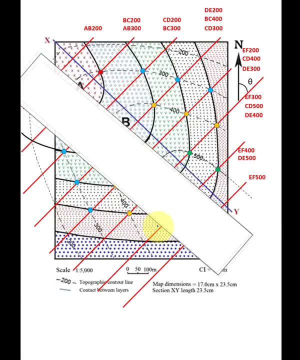 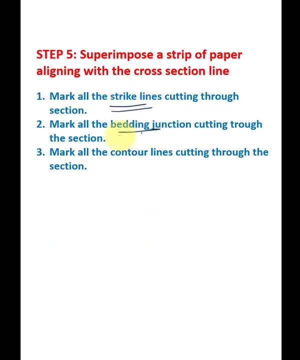 You have to align it like this And what you have to mark is just see what all things we need to mark, Mark all the strike lines, Mark all the bedding junctions and mark all the contour lines. So strike line, bedding junction, contour lines. 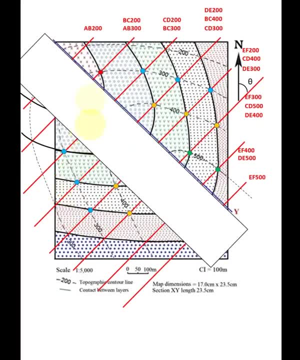 These three things we need to mark on this strip. So first strike lines are these red color ones. Before that, let us first mark our x and y. So these two points are very important. Only between these two points, All of them, All the other points will lie. 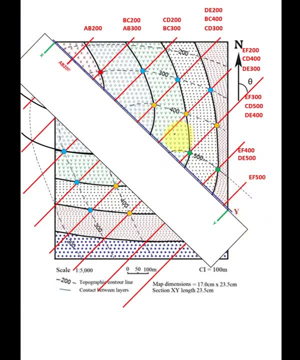 So first you should always mark your x and y, Then we need to mark all the strike lines. So wherever the strike line is cutting or wherever the strike line you are getting on the strip of paper, you just have to mark it and you will have to write the name of that. 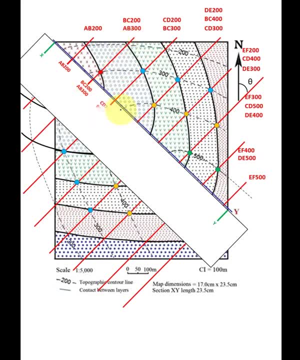 strike line also. Okay, This is very important, This strike line: CED 200, BC, 300, then this one, Okay, all the names. Then there is this strike line, Then here this one and finally this one. So all the strike lines. we have marked it on the strip of the paper. 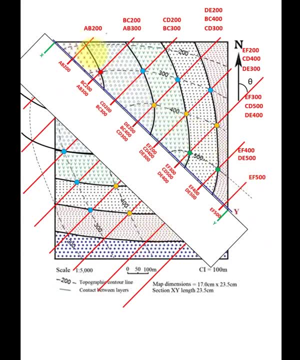 Next was we need to mark all the bedding junctions. What are the bedding junctions? These one? the black, solid black lines. So first bedding junction is AB right. Next we get here a bedding junction which is BC. Next we get bedding junction CD, DE. 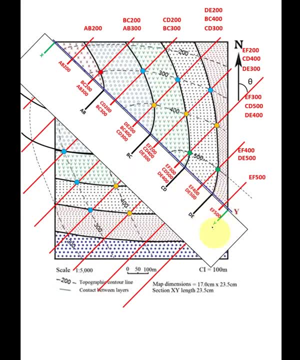 Right. Next, we get here a bedding junction which is BC Right. So these are the bedding junctions which we come across this line XY. Then we need to mark the contour intervals, right. So first contour interval you get here which is cutting that XY. 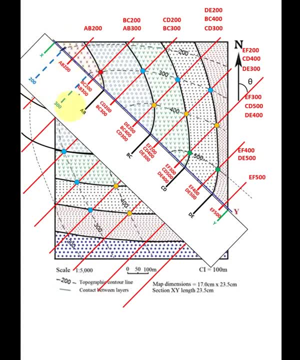 So it is 200.. Next you will get here which is 300.. Next is this one which is 400.. Next is this one which is 500.. And any other contour interval? I don't think so right, no other contour interval. So this is basically all the markings that we have done. 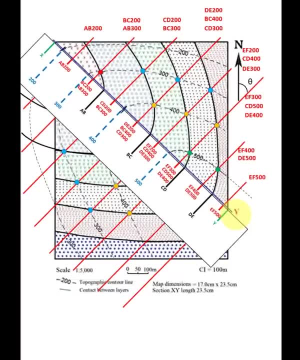 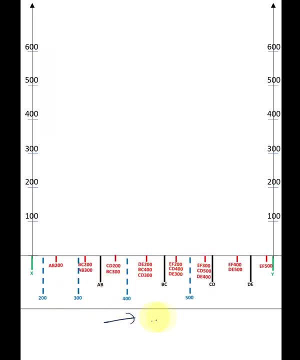 Now we need to plot the strike lines. So what you have to do, this strip of paper that you have right now. you will use that strip of paper as the X axis, Okay, Okay, Okay. So this is the strip of paper as the X axis and the vertical axis you will mark, same as. 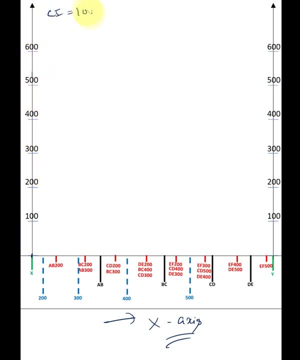 your contour interval. So your contour interval was 100 meters, right. So you will draw two vertical axis from the X and Y points- X and Y points- and you will mark a scale of equal to your contour interval, Okay, Which is 100.. 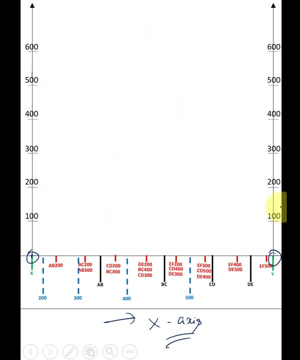 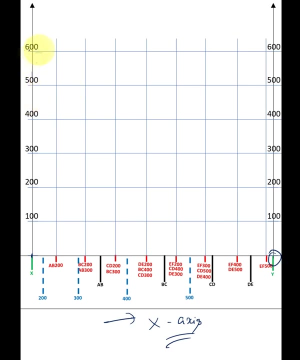 Okay, Okay. So this is the plot where we are going to draw the actual cross section of the map. So now what we need to do is we need to first draw all the lines like this. So first it will be through all these points, points of elevation. 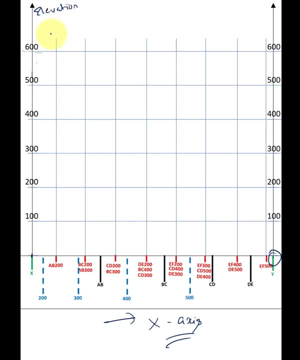 So this is elevation, Okay, This is your elevation. and on X axis you have your horizontal length along the XY, Okay, Okay. So from these strike lines we will be having our vertical lines going and from these elevation points we will be having the horizontal lines going. 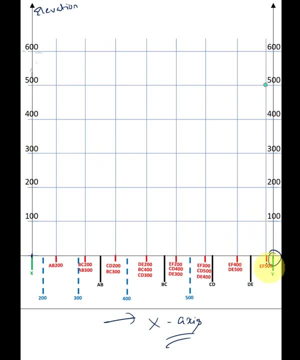 What you have to mark is now: first you mark this 500 point, EF 500.. So at every strike line you will have to mark all the points. So EF 500, since it is having the elevation of 500, you will mark here at 500.. 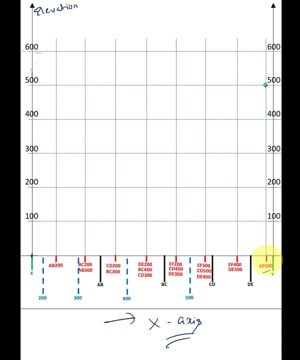 Okay, The one which is intersection of EF and 500. you will mark that point. Next we have EF 400 and DE 500.. So first what we will do is we will mark all the points of one strike line, that is, EF. Then we will start with DE. 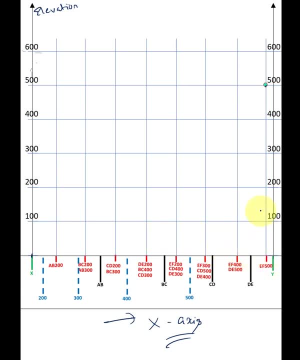 Then we will start with CD That way. Okay. So first let us finish marking all the points of one of the strike lines: EF, So 500 is the one, Then EF 400, which will be the intersection of vertical line from this EF and horizontal. 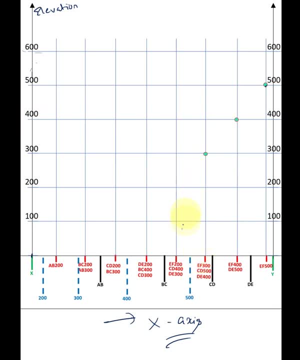 line from the 400. Then EF 300. Then EF 200 is there, That's it. So these are all the points of your EF. We will draw a line through all these points and this is the bedding junction EF that you have drawn. 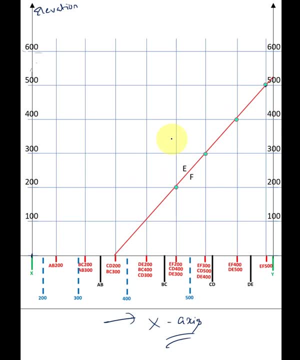 Basically Okay. So this is your EF. Okay, This is your bedding junction EF. Next, we will come to the next strike line, which is DE. So DE 500 is there. So, from this intersection of DE and 500, we will plot one point here: 500. 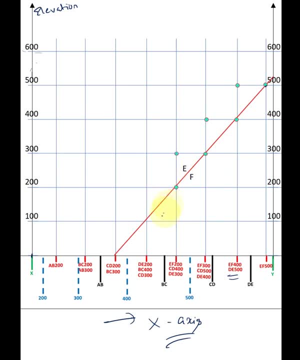 Then we have DE 400 here, Then we have DE 300 and finally DE 200, and we will again take a line through them. This is your bedding, junction DE- Okay. After that we have CD. So CD 500 is there. 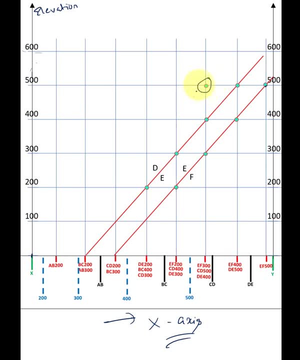 So vertical line from CD and 500. we get this point, Then CD 400, CD 300 and CD 200. So we will just plot a line through them. We will get a bedding junction, CD. Next we have BC. So BC 400 we have. 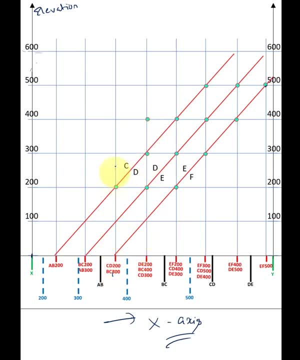 BC 400.. Then we have BC 300- this point- Then we have BC 200- this point- and we will draw a line through it. That would be your bedding junction, BC. Next, we have AB 300 and AB 200.. Okay, 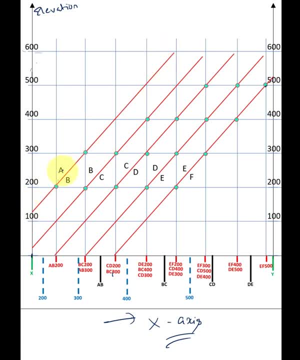 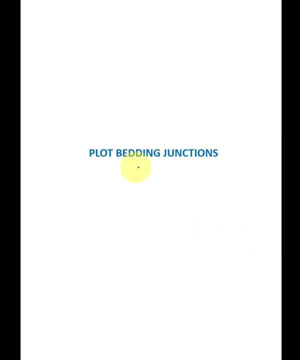 So we will pass a line through it. That will be our AB bedding junction. Now what you need to do is, after plotting all the strike lines, we need to plot the bedding junctions. So what I mean by plotting the bedding junction is: see, I will show you. 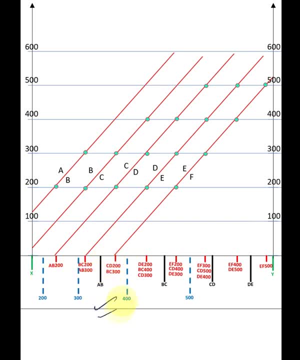 Now we have bedding junctions also on this strip of papers. See, these red color things were your strike lines. These dark black things are your bedding junctions. I will just write: Okay, So these are your bedding junction junctions and these dotted lines are your contour lines. 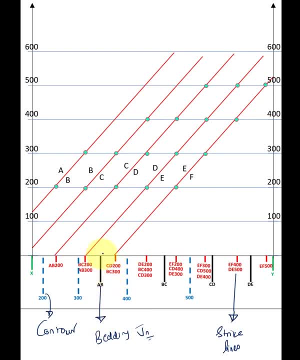 Okay, So these bedding junction AB. what we have to do is that we have to take a vertical lines from this AB and we need to mark it on the bedding junction AB here. This is your AB, So we have to take a vertical line from here and we need to mark a point. 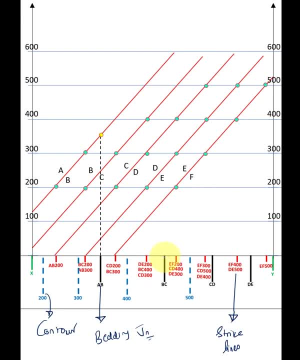 Alright, Same way We will do it for BC also. BC. the bedding junction here is this, This one, This is the bedding junction, So BC where it intersects on that bedding junction. This is the point. I have marked it with yellow. 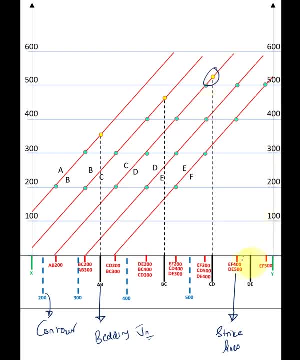 CD on this CD junction here and DE on the DE junction here. So you need to understand that. why have we drawn these bedding junctions on these red lines, Red bedding junction lines? The thing is that you need to understand that this view, what you are seeing, of the 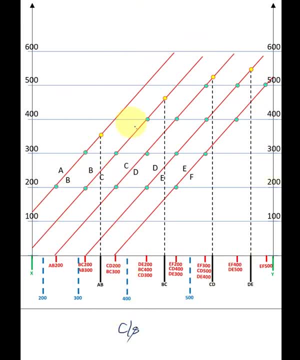 map. this is a cross sectional view and the question that was given to you was a top view. Right, You were seeing it from this point and from the top view. those dark lines that you saw as bedding junction lines, these were actually these lines. Okay, 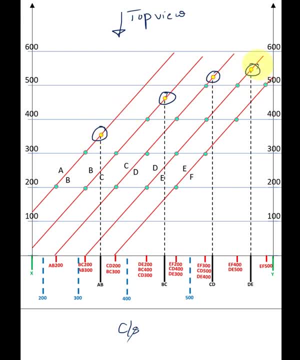 These points that we have drawn here. Of course, in a cross section it would look like a point, But from top view, From top view, it would look like a line. I hope you can imagine it. When we cut a section through it. definitely a line cannot be shown in a section. 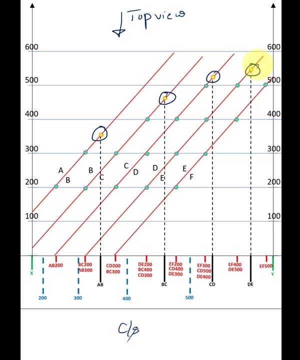 A line will be looking as a point, But from the top view we understand that these are basically our bedding junctions as dark lines. The next what we need to plot is the contour lines. So these dotted lines that we know they are contour lines. 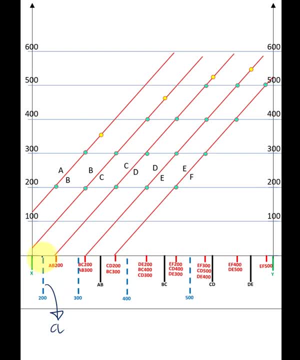 So these dotted lines would be Like: if here we are starting with 200, we just simply have to take it till 200, that's it. So here I mark one point: this: 300 will go till 300, then 400 will go till 400, 500, that's. 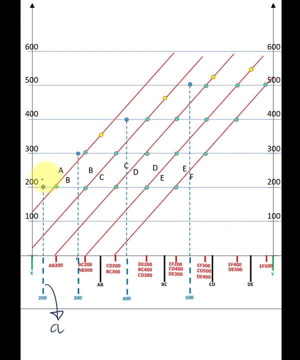 it. So now, basically, what you have got is the points which you need to connect, and the points that you need to connect are these blue points and the yellow points. Okay, These are the points that you need to connect And that will complete, basically, your cross section. 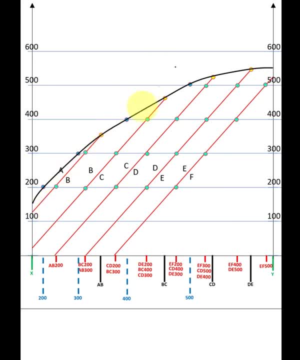 So when you connect them like this and you erase the top part, this is nothing but the cross section of your map. That's it And this entire thing, that you see this area. this is your F plane. This is your E plane. This E and E will become a E plane. 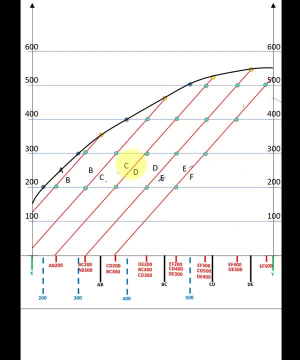 Similarly, This D and D will become a D plane. This is a C plane, B plane and A plane. Okay, and when you see from the top, this is like your A, B, C, D, E, F and these were your. 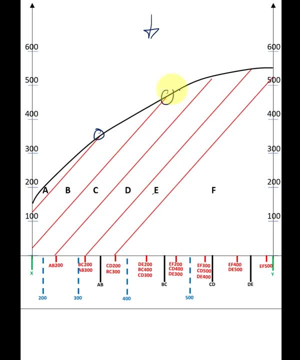 bedding junctions. This one, this one, this one and this one is what you were seeing from the top view. Alright, So this is your basic cross section of your first map, Which is the easiest map of them all. In the other maps we will be also doing fault, fold and unconformity, I guess.